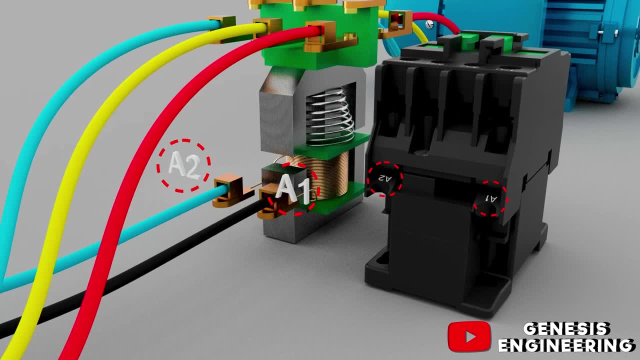 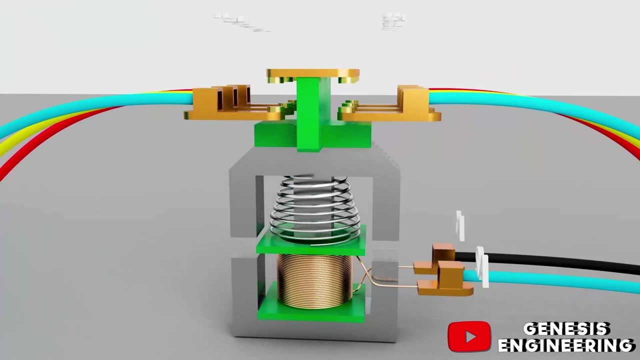 Now we connect one phase to A2 and neutral to A1.. Basically, the contactor will work as follows. Inside the contactor we have the core, which is made of a ferromagnetic material, which is divided into two parts: a mobile core and a fixed core. 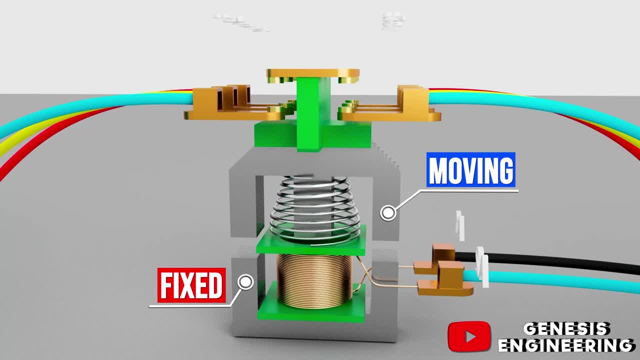 With the contactor de-energized, the moving core is forced upward by a spring Spring pressure causes the contacts to be open while the contactor is de-energized. For the contactor to start working, it is necessary to energize its coil, which are contacts A1 and A2.. 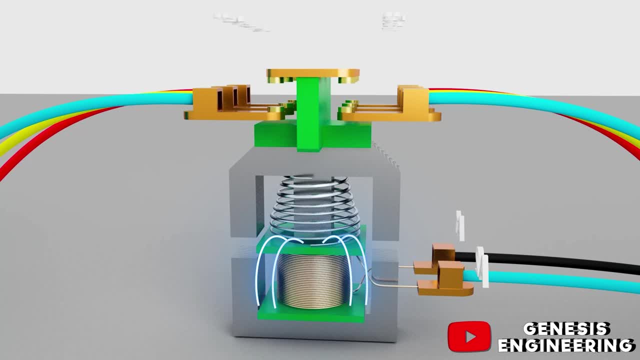 When your coil is energized, an electromagnetic field is created around it. The electromagnetic field produced by the coil ends up surrounding the fixed core and it ends up attracting the moving core. In this way, the contactor will close the contacts and start the motor. 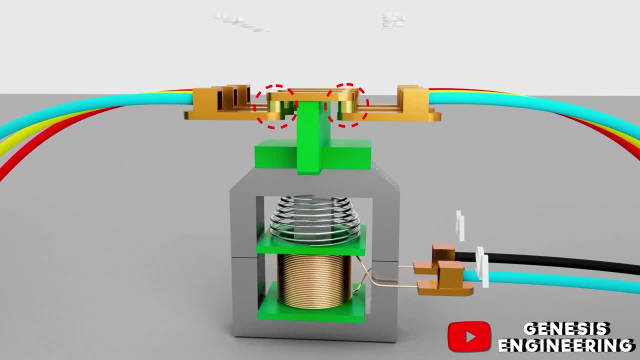 If the power is turned on, the contactor will be energized. If the power supply is turned off at the coil terminals A1 and A2, the contactor will open the contacts and stop the motor. We understand how the contactor works now. Why is it used? 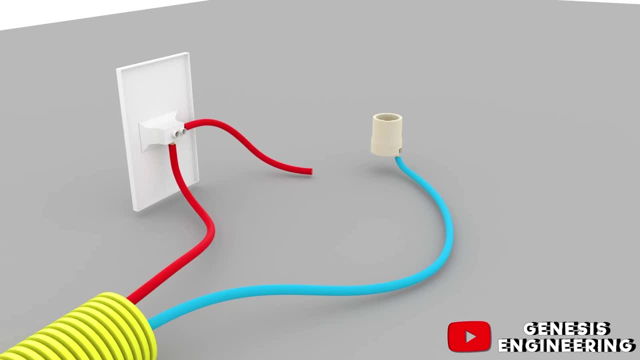 Inside the residence. to be able to turn a lamp on and off, a simple switch is used to be able to activate it. Now, in the case of a motor, to be able to turn this motor on and off, we need a device that supports higher currents, and for that we need a contactor. 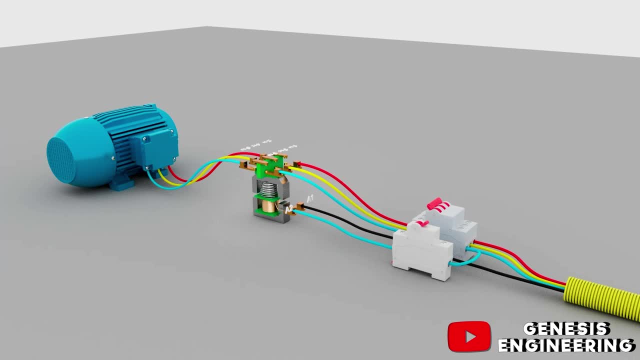 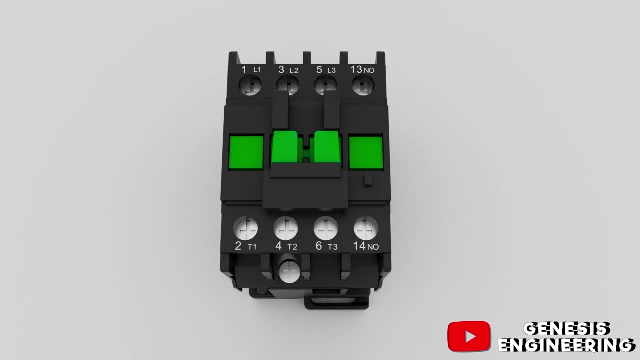 The contactor will allow the control of loads with high currents in a safe and efficient way. Remembering folks that I made this simple connection just to be able to better explain how the contactor works. Now, to start and stop the motor, it is necessary to use buttons, and to use these buttons, auxiliary contacts 13 and 14 of the contactor are used. 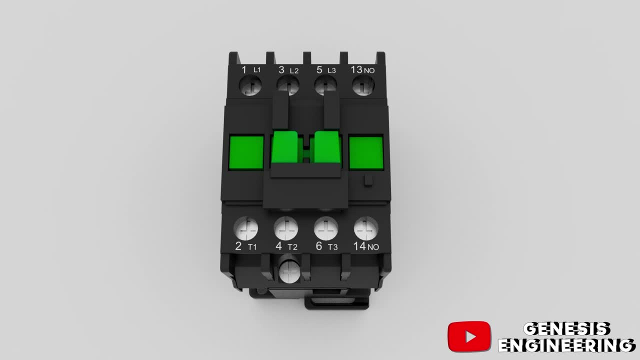 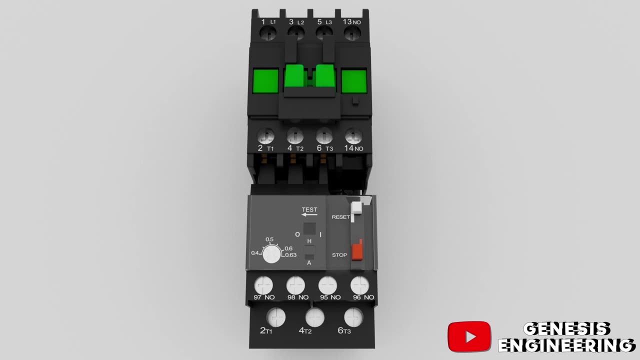 To protect the motor, it is necessary to use a thermal relay together. What do you guys think of continuing the videos about contactor and electrical controls? comment below on the video, already leaving your like to help our channel grow. thank you very much for watching and until the next video.